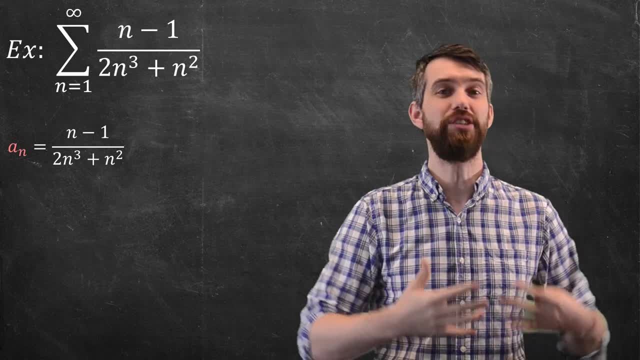 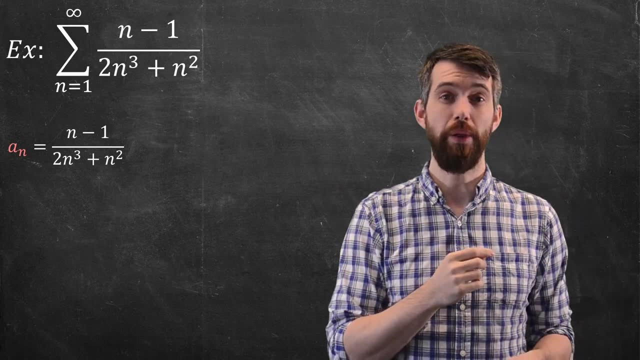 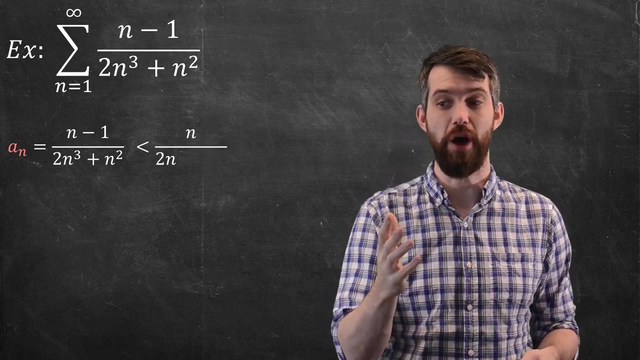 Well, let me consider the ANs here, this expression, and let's try to do a comparison with something that's a little bit nicer. Indeed, if I look at the numerator, if I look at the N-1 here, well, the numerator- because I subtract 1, is strictly greater than if I have the same denominator but only N on top. 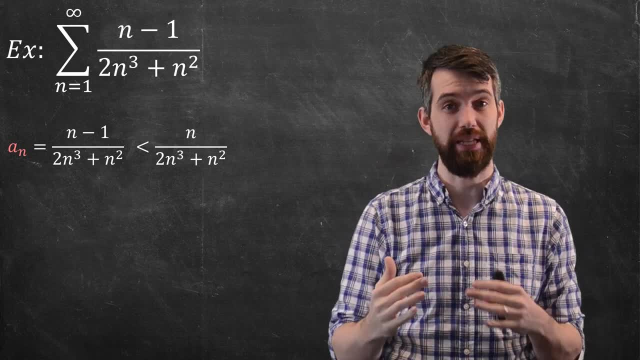 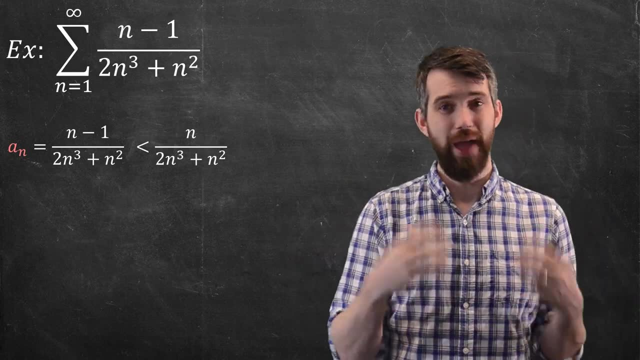 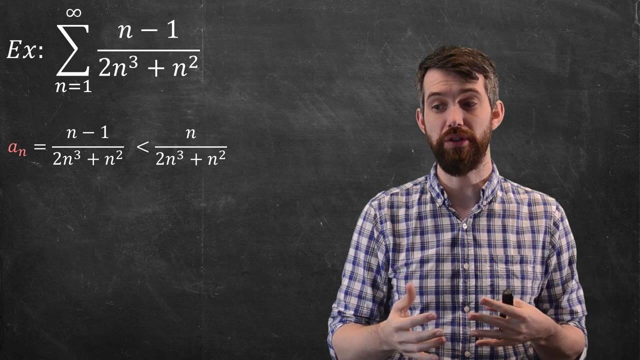 As in, this is less than N over 2N cubed plus N squared. And then if I focus my efforts now on the denominator, well, in the denominator I have this plus N squared. N squared is something positive, so the positive in the denominator makes the entire thing smaller. 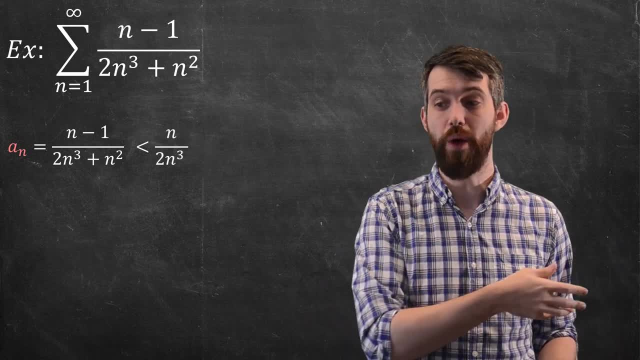 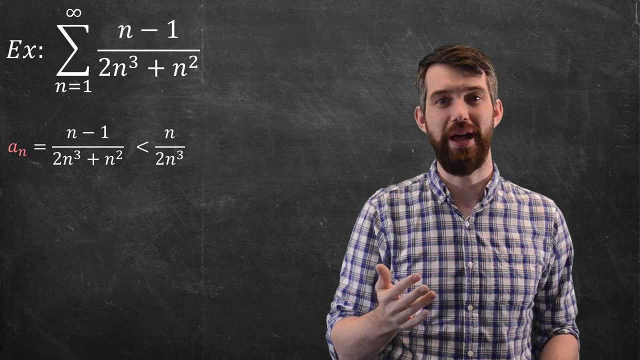 So it's also going to be smaller. if I just take away that N squared and just write it as N over 2N cubed, This is a strict inequality. And then N over N cubed, I can cancel out one copy of N and I'm just left with 1 over 2N squared. 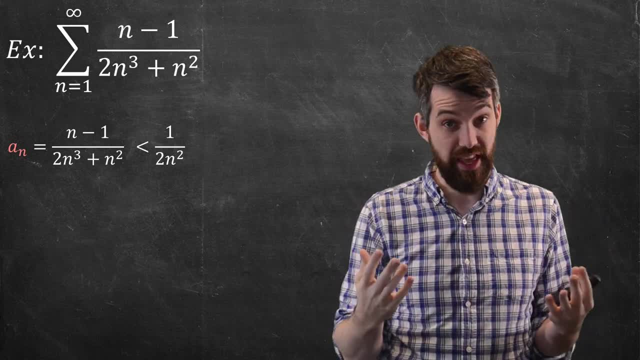 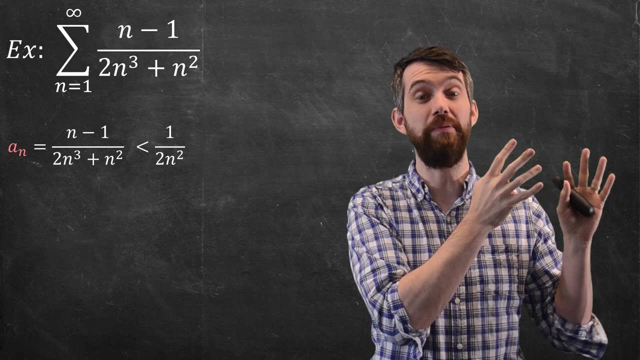 So I have this inequality that's taken, this messy thing, the AN that I didn't like. so I have this inequality that's taken, this messy thing, the AN that I didn't like, and I've related it to a BN, which is much simpler. 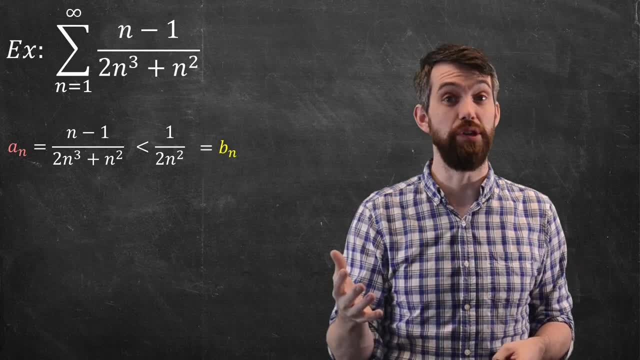 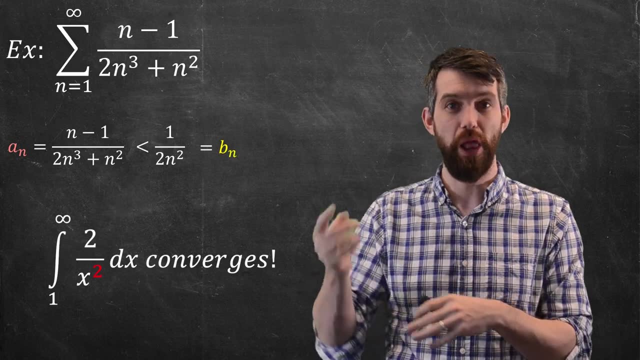 In fact I know whether this BN converges or diverges. It is a P-series. Back when we did the integral test, when we compared it to the P-integral, the improper integral 1 up to infinity of 1 over X squared. 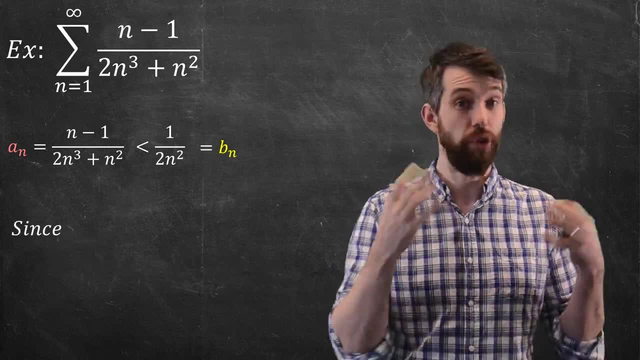 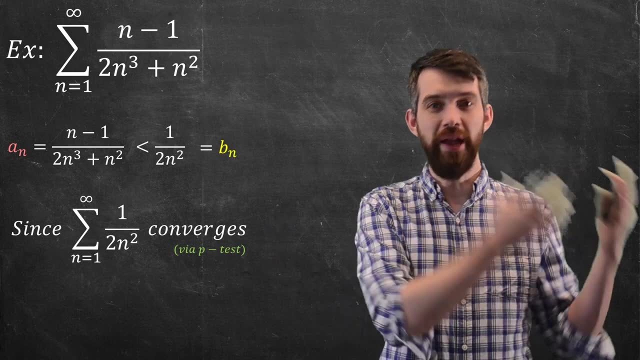 that converged because the P of 2 is greater than 1.. So, indeed, we know that the sum of this 1 over 2N squared the BNs, that converges by the P-test. And if this bigger thing converges, 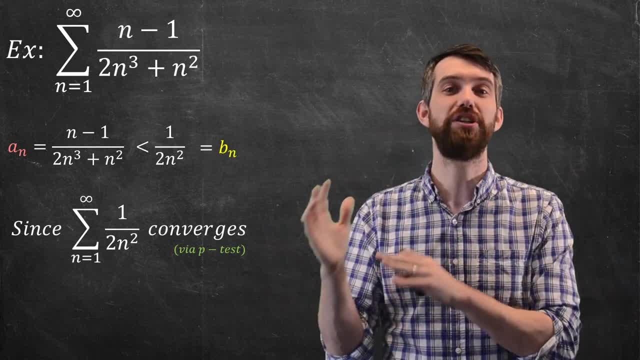 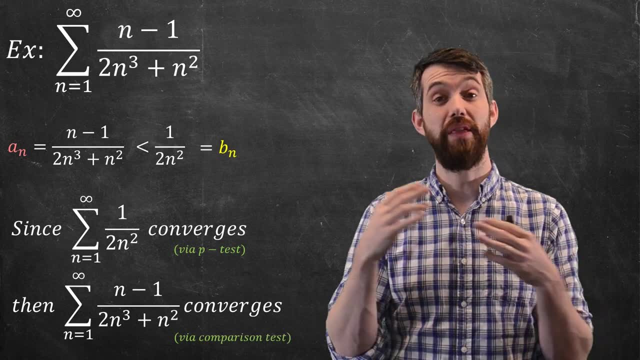 then the smaller ones. the sum of the ANs has to converge as well. So what do we get? We get that this summation indeed converges too. Notice, by the way, that because I demanded that the ANs and the BNs were both positive, 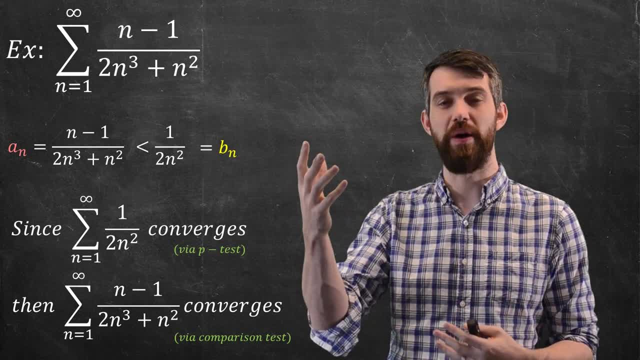 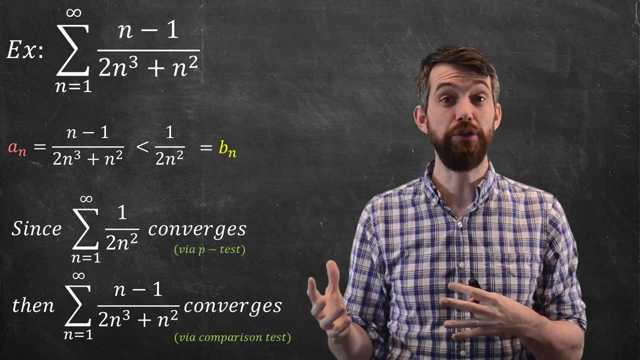 that meant that you didn't have some scenario where the bigger one converged but the smaller one went down to minus infinity. Going down to zero was the smallest it could be, So this comparison test is really useful for converting series that are messy and complicated. 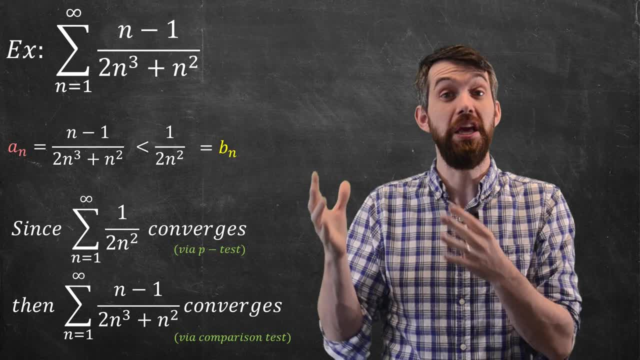 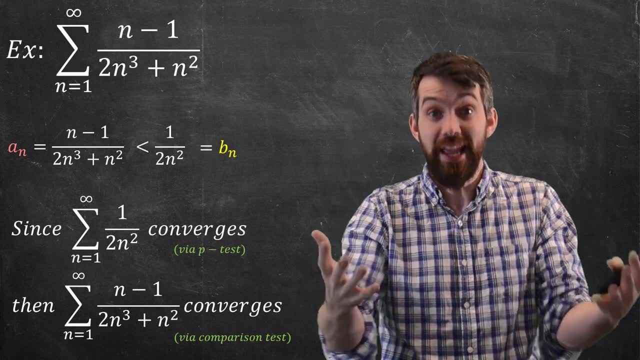 and we don't want to deal with into much simpler ones where, hopefully, we already know the answer to whether it converges or whether it diverges. Notice, by the way, that it doesn't converge to the same thing.